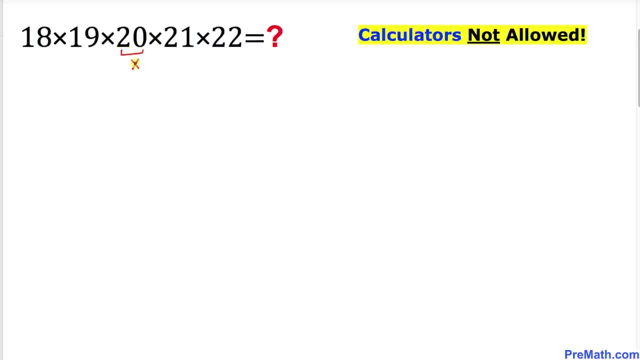 this middle number, 20 as an x. so that means let's say that x equal to 20. then this number is going to become x minus 1. this number is going to become x minus 2. on the other end, this number is going to become x plus 1 and this number is going to become 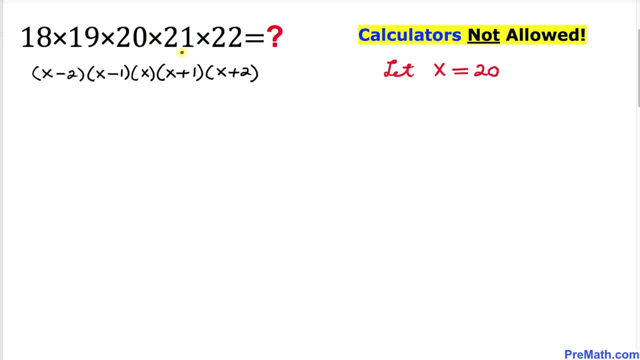 x plus 2.. So, therefore, I wrote down 20 as an x, 19 as x minus 1, 18 as x minus 2, and here 21 as x plus 1 and 22 as x plus 2. and here's our next step. Let's go ahead and rearrange these numbers. I am going to put x minus 1 and x plus 1 together, and 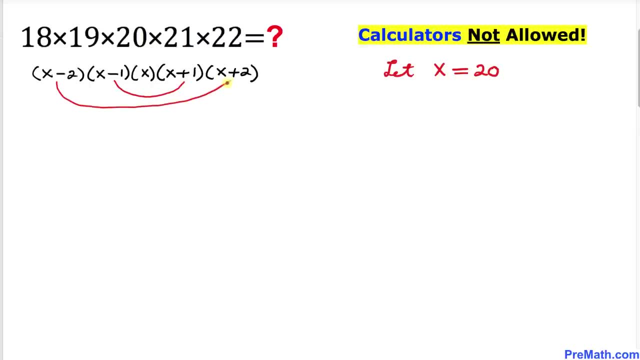 likewise x minus 2 and x plus 2 together. So therefore I can write it as x, and then times x minus 1 times x plus 1, and likewise x minus 2 times x plus 2, and now let's focus on these two factors. 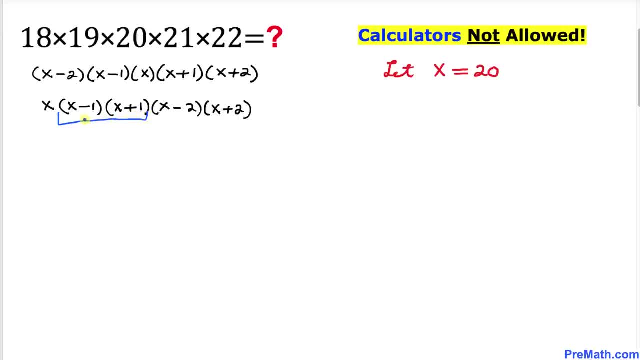 minus 1 and x plus 1. we are going to use this formula. so therefore, this part could be written as: x square minus 1, square, which is same as x square minus 1 square is same as 1, and likewise- let's focus on this part over here- these two factors: x minus 2 times x plus 2. we are going to use this. 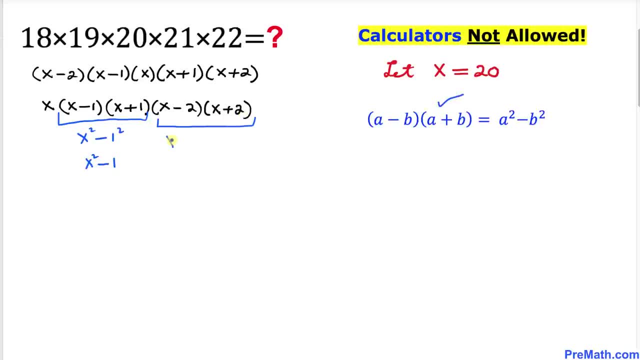 formula once again. so this could be written as x square minus 2 square, which is same as x square minus 4, so therefore we can write this one as x times x square minus 1 times x square minus 4. and now let's focus on these two factors. 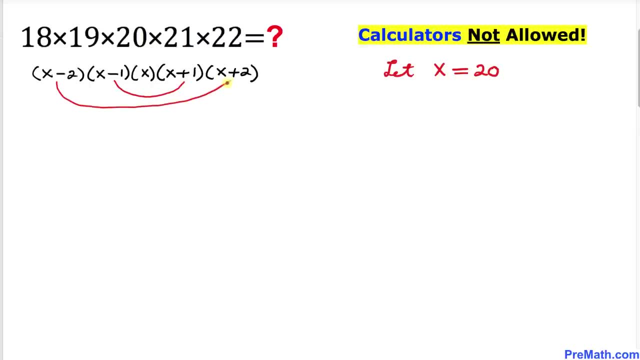 likewise x minus 2 and x plus 2 together. So therefore I can write it as x, and then times x minus 1 times x plus 1, and likewise x minus 2 times x plus 2, and now let's focus on these two factors. 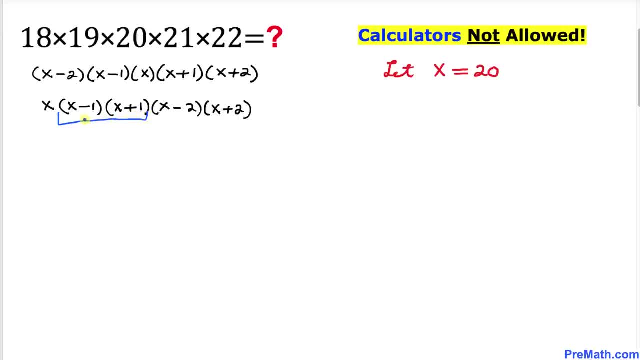 minus 1 and x plus 1. we are going to use this formula. so therefore, this part could be written as: x square minus 1, square, which is same as x square minus 1 square is same as 1, and likewise- let's focus on this part over here- these two factors: x minus 2 times x plus 2. we are going to use this. 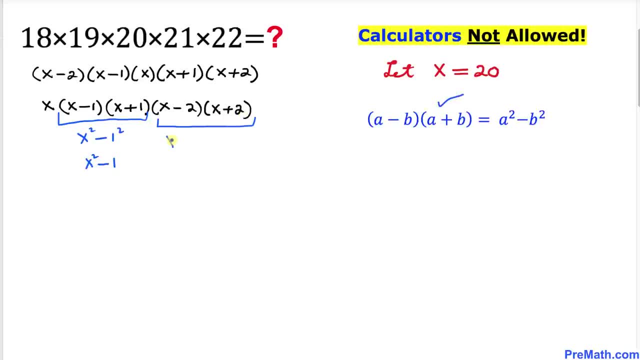 formula once again. so this could be written as x square minus 2 square, which is same as x square minus 4, so therefore we can write this one as x times x square minus 1 times x square minus 4. and now let's focus on these two factors. 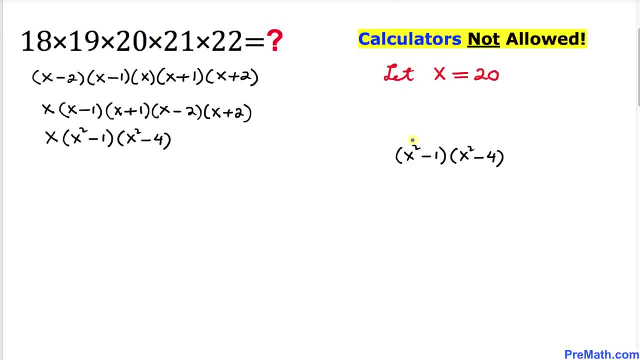 and here I have copied them down. and now let's go ahead and do the double distribution and then we're going to multiply them. so this is going to become x power 4 minus 4 x square, minus 1 x square, and then plus 4. let's combine the like terms x power 4 and this is going to give us negative 5x square minus 4 x square. 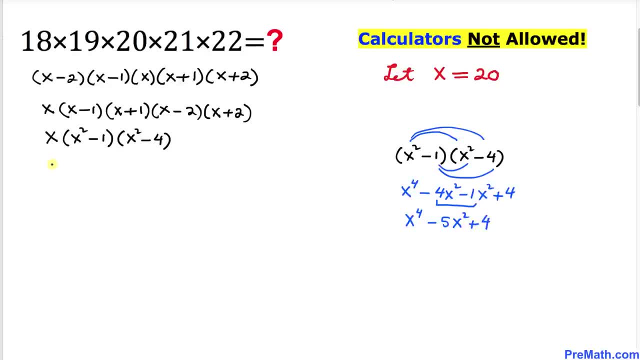 plus 4. so therefore we can write this one as x time x: power 4 minus 5, x square plus 4, and now we know that our x value is 20. so wherever we see x, I am going to replace each of these one by 20. so therefore I can write this one as 20 times: this is 20, and then power 4. 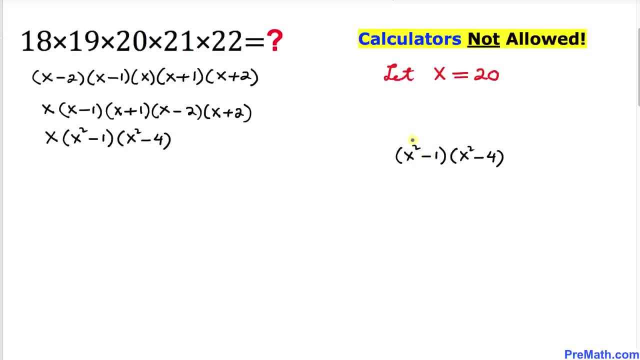 and here I have copied them down. and now let's go ahead and do the double distribution and then we're going to multiply them. so this is going to become x power 4 minus 4x square, minus 1x square, and then plus 4. let's combine the like terms x power 4, and this is going to give us negative 5x square. 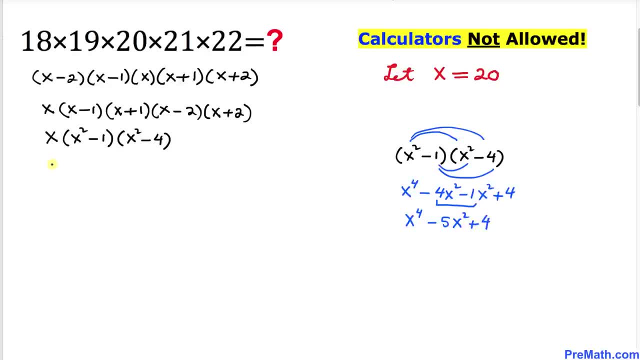 plus 4. so therefore we can write this one as x time x: power 4 minus 5, x square plus 4, and now we know that our x value is 20. so wherever we see x, I am going to replace each of these one by 20. so therefore I can write this one as 20 times: this is 20, and then power 4. 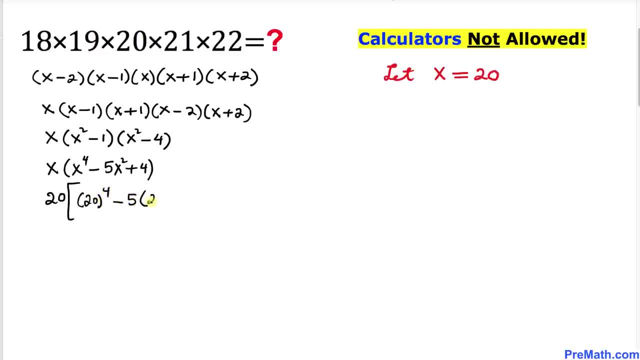 minus 5 times 20, and then square, and then plus 4, and now we are going to simplify this, and now let's focus on this part: 20 power 4, and here I have copied down 20 power 4. and now this 20 could be written as 2 times 10, and then I just separated them, so this: 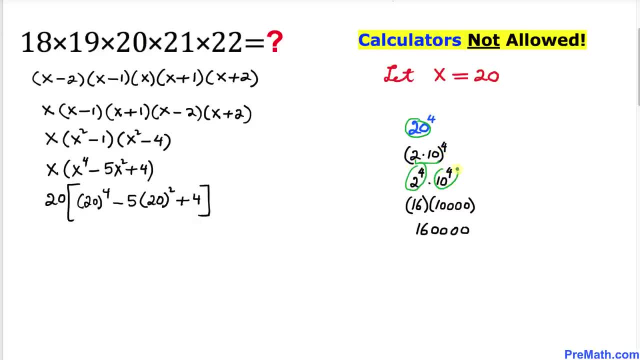 could be written as 2 power 4 times 10 power 4. 2 power 4 is same as 16 and 10 power 4 means we are going to put four zeros and if we multiply them we are going to get 16 with the four zeros. 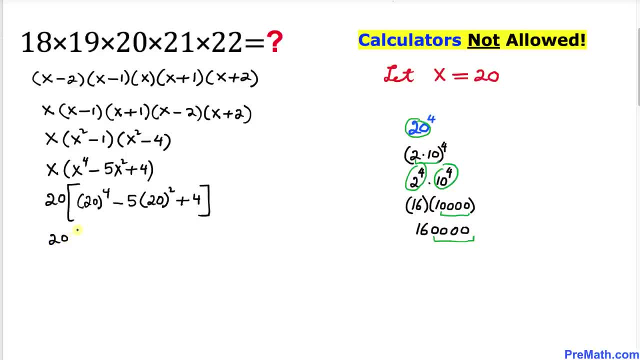 so, therefore, we can write this one as x power, 4 minus 5, x square plus 5, x square plus 4, and we are going to put 4 versus 4.. Now, let's do this. Now, thisect this one: 20, out side the bracket, and this could be written as 120 and 60 thousand, and then 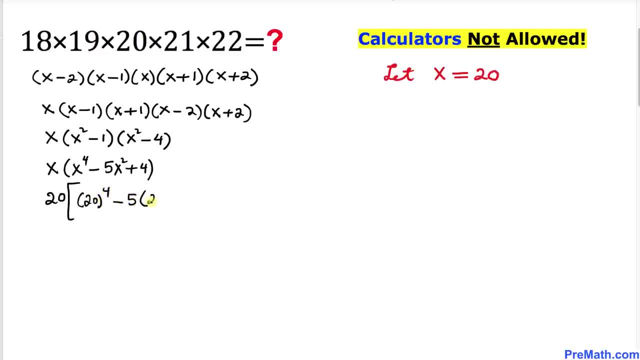 minus 5 times 20, and then square, and then plus 4, and now we are going to simplify this, and now let's focus on this part: 20 power 4, and here I have copied down 20 power 4. and now this 20 could be written as 2 times 10, and then I just separated them, so this: 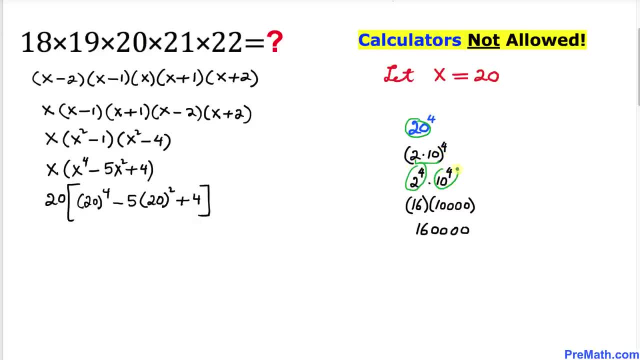 could be written as 2 power 4 times 10 power 4. 2 power 4 is same as 16 and 10 power 4 means we are going to put four zeros and if we multiply them we are going to get 16 with the four zeros. 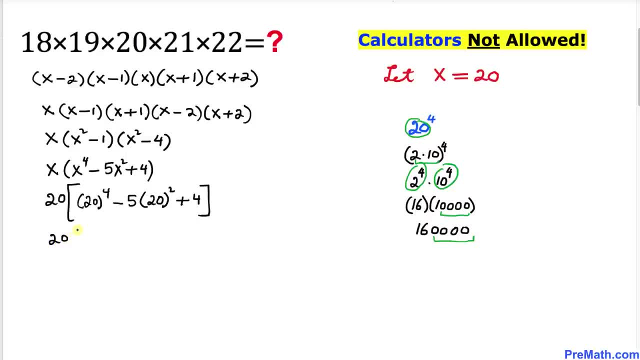 so, therefore, we can write this one as x power, 4 minus 5 x square plus 5, x square plus 4, and this one 20 outside the bracket, and this could be written as 160,000, and then minus 5 times this. 20 square is same as 20 times 20 is 400, and then plus 4, and now, in this next step, 5 times 400. 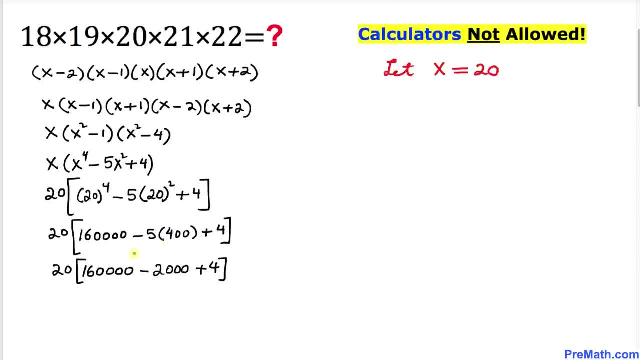 is going to give us 2000. and now let's focus on these numbers inside this bracket- and here I have copied them down- and we can see that 160,000 minus 2000 is going to give us 158,000, and then plus 4, so they add up to 158,004. 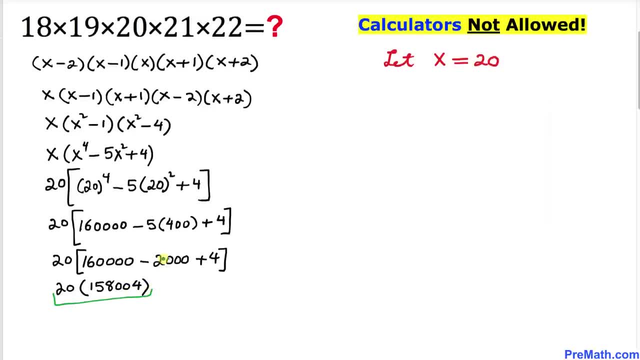 now let's focus on these numbers, and here I have copied them down. and now I have broken down this 20 in to 10 times 2, and then I multiplied 2 times of this number, 158,004, and that gave us 316,008. 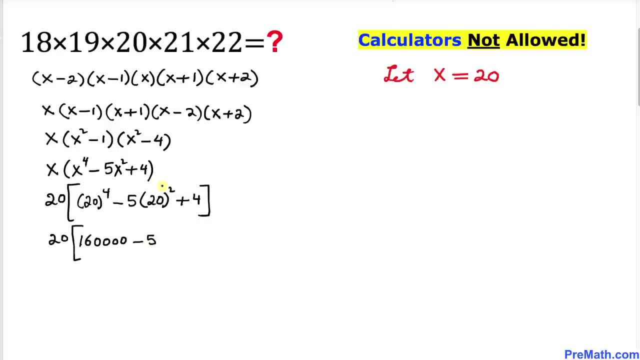 minus five times this, 20 squared is same as 20 x 20 is 4 hundred. and then plus four, and now, in this next step, five times 404.5 x 4xit's very easy. We will Mand at 4: 4. I am going to put 20 outside the bracket, and this could be written as 160, thasnd, and than minus 5 times this, 20 squared is same as 20 times 20 is 400. and then plus 4. and now, in this next step, 5 times 40 Fr, plus 2, and now, in this next step, 5 times 40 Fr. and now, in this next step, 5 �tani years, four hundred an. 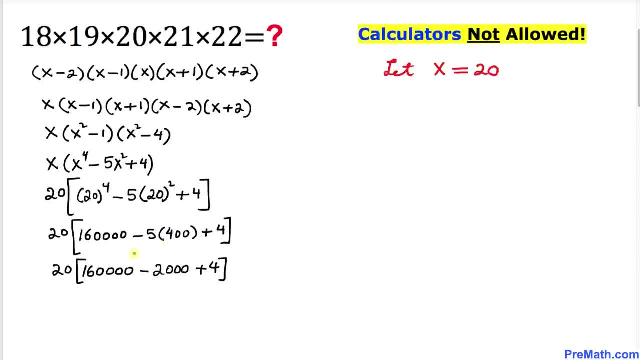 is going to give us 2000. and now let's focus on these numbers inside this bracket- and here I have copied them down- and we can see that 160,000 minus 2000 is going to give us 158,000, and then plus 4, so they add up to 158,004. 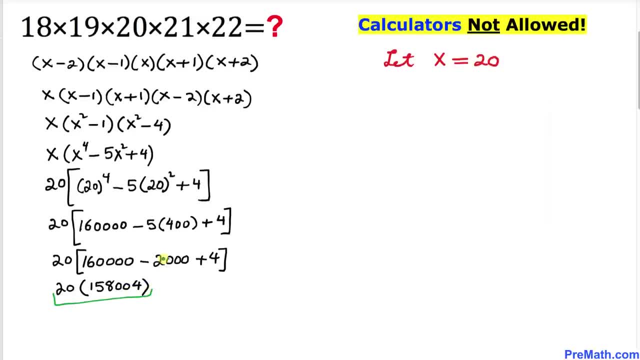 now let's focus on these numbers, and here I have copied them down. and now I have broken down this 20 into 10 times 2, and then I multiplied two times this number, 158,004, and that gave us three hundred and sixteen thousand and eight. 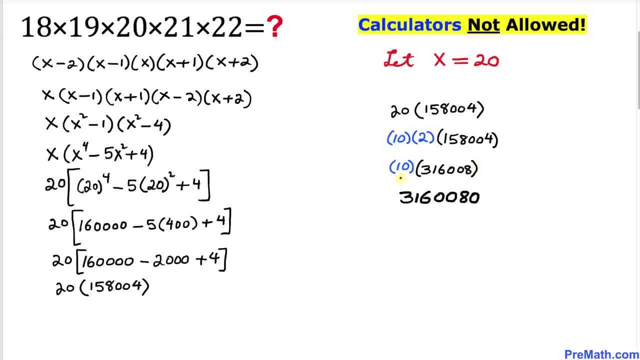 and finally, I multiply this number by ten, so we got 3,160,080.. So thus we got our answer as 3,160,080.. And that's our final answer. Thanks for watching and please don't forget to subscribe to my channel for more exciting videos. Bye.